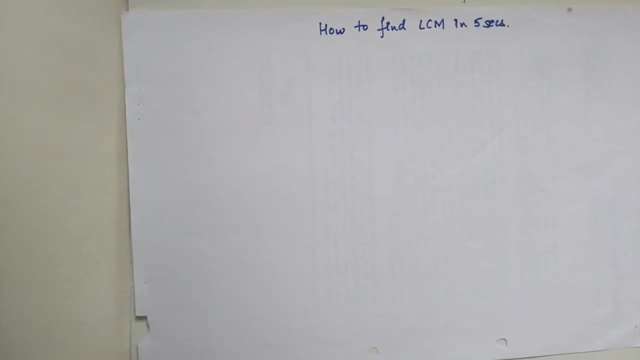 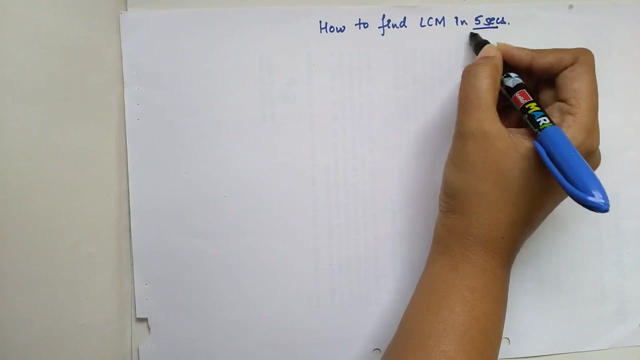 Welcome everyone. So today, in this video, I'm going to show you how to find the LCM of any given set of numbers in matter of five seconds. But before beginning with that, students, I would like to thank all of you all for all your likes, subscribes and shares. 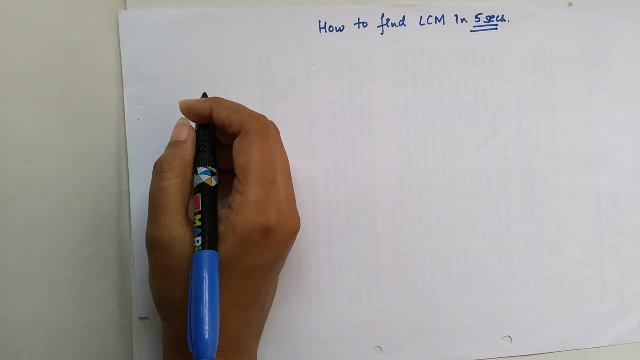 And if you're new to my channel, then do hit the subscribe button and also the bell button so that you will get notified whenever I post a new video. Also, students, I would like to remind all of you all: this channel is purely created with the intent of giving tricks and tips, as well as solving your doubts. 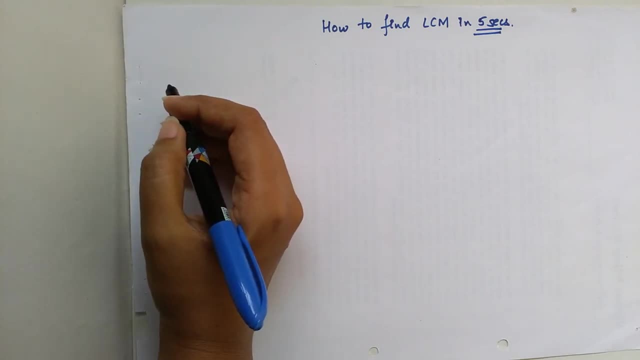 So if you have any doubts, then please put those in the comment section, or you can email me so that I can make a video for you and all the others also can get benefits from you. So let's begin with our video. So, students, what do I mean by LCM? 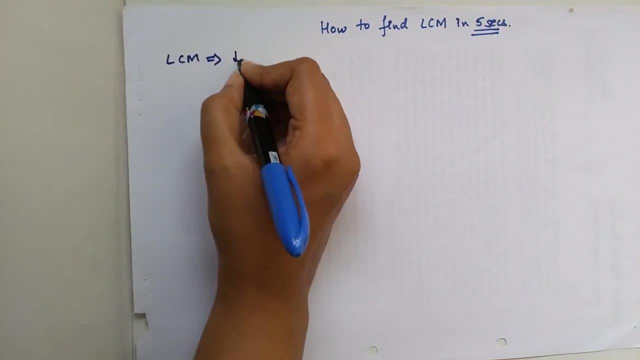 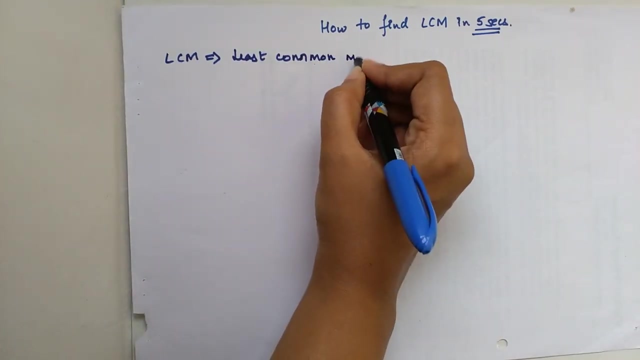 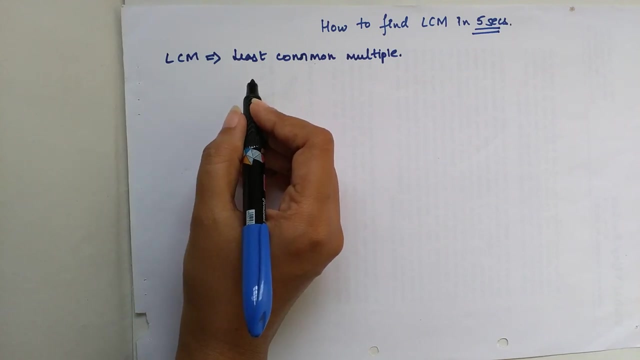 LCM actually stands for least Common Multiple, Meaning that you need to find a number which will be a multiple of all the other given numbers. So now let's take, for example, numbers are like 4,, 8 and 16.. 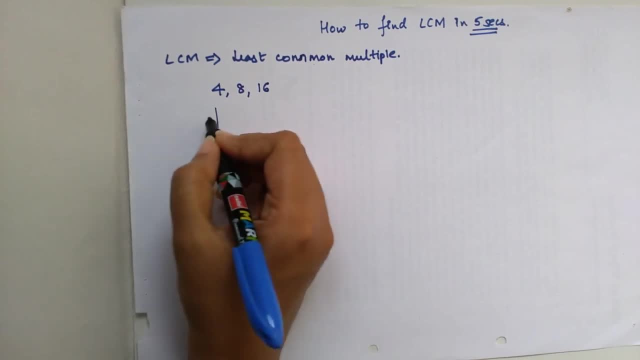 So, students, the traditional method was just write all of them: 4,, 8 and 16.. And then you start writing their prime factors. So here we do 2.. So we get 2,, 4, 8.. Again 2.. 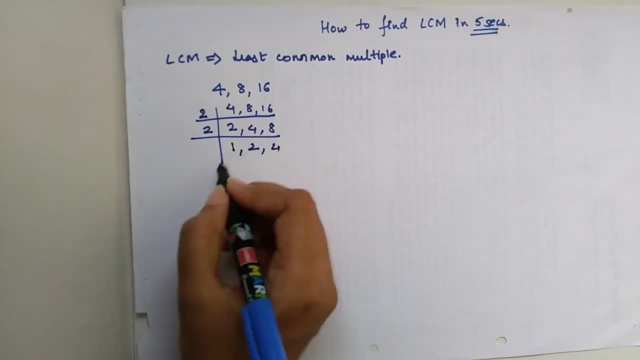 We get 1, 2 and 4.. Again, we take 2.. We get 1, 1 and 2.. And one more 2 gets us the answer 1, 1 and 1.. So this method you need to continue until and unless you get all 1s over here. 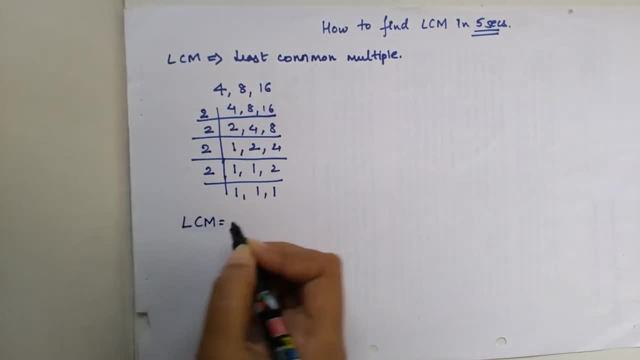 So from here we can say that LCM is equal to 2 into 2, into 2 into 2, which is equals to 16.. But this method is quite lengthy, especially when we're talking about entrance exams. Also, in our normal exams, if we need to find out the LCM and if we use this method, it might be a bit time consuming. 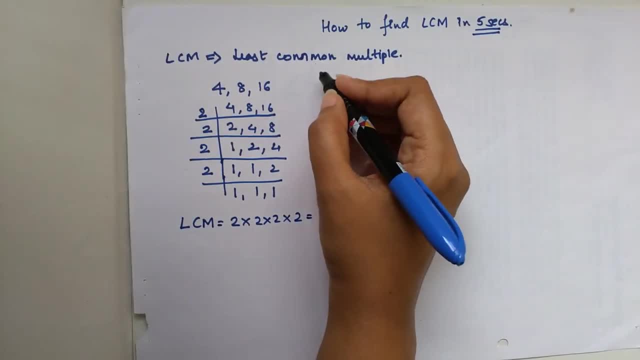 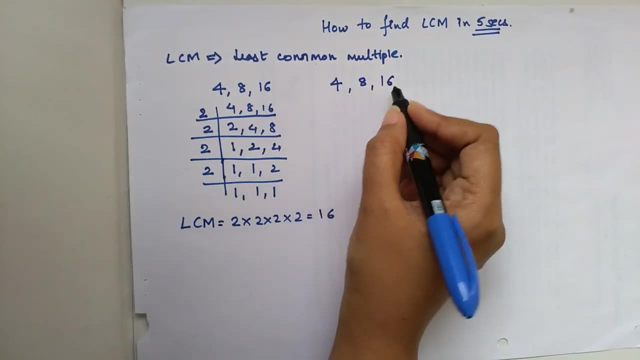 So over here I'm going to show you a trick. So let us take these numbers again: 4,, 8 and 16.. The trick is very simple. All you need to do is you need to take the highest number from the given set of numbers. 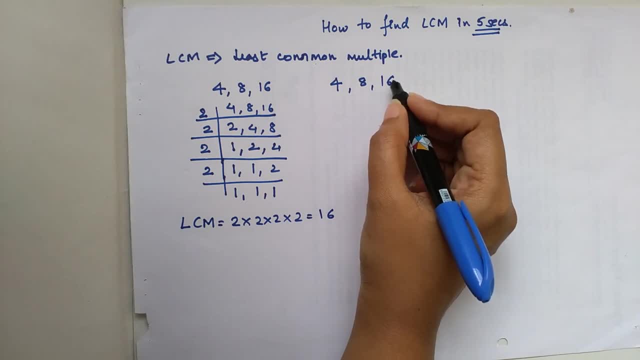 So over here, 16 is the highest number. So now, what do we need to do is we need to check whether 16 is a multiple of 4 and 16 is a multiple of 8.. In simple terms, we need to check whether 16 comes in 4 tables and whether it comes in 8 tables as well. 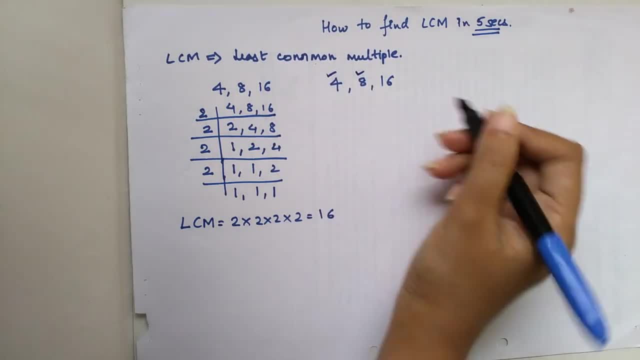 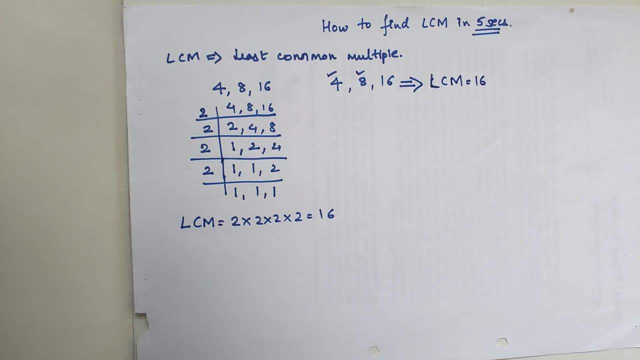 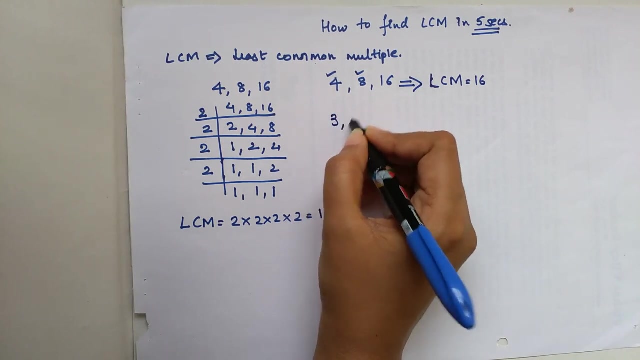 So, as we know, 4- 4s are 16 and 8- 2s are 16.. So here my LCM Is equals to 16.. OK, now let us take a different example. So the number is 3,, 4, 6 and 18.. 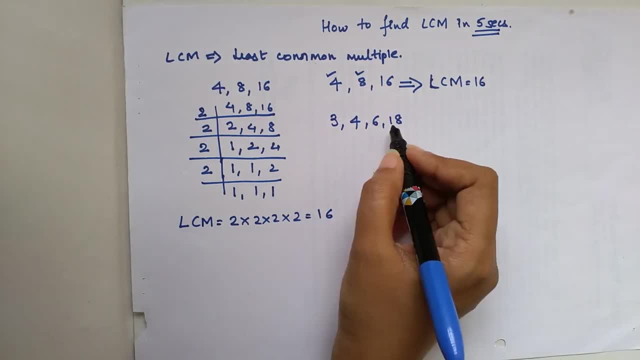 Now let's see what is the highest number. The highest number is 18.. And we need to check whether 18 comes in the table of 3, 4 and 6.. So over here we can say that it doesn't come in the table of 4.. 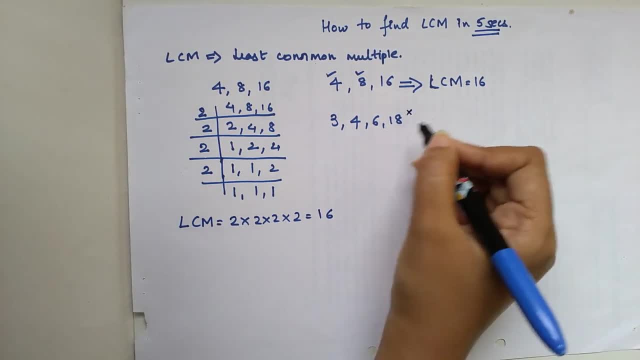 So the next step which you would do is you will simply multiply the highest number, that is, 18, by 2.. Once you multiply 18 by 2, the number you get is 36.. Now you will be checking whether 36 is a multiple of 3,, 4 and 6.. 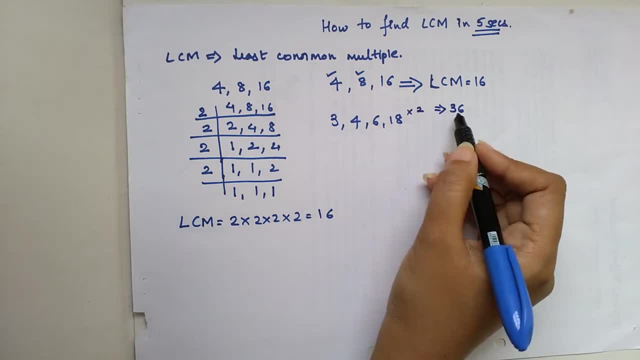 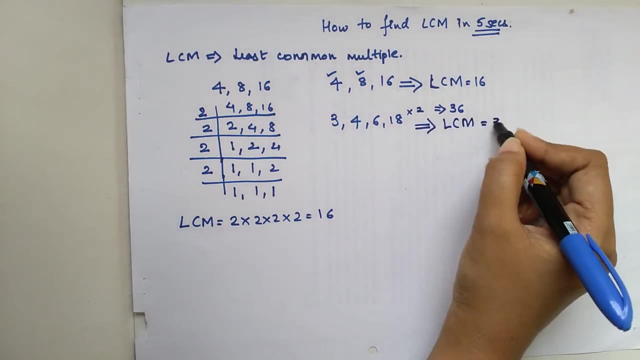 So, as we know, 3- 12s are 36,, 4- 9s are 36 and 6- 6s are 36.. So here now, my LCM became 36.. Now let's see what will be the LCM of 5,, 10,, 15,. 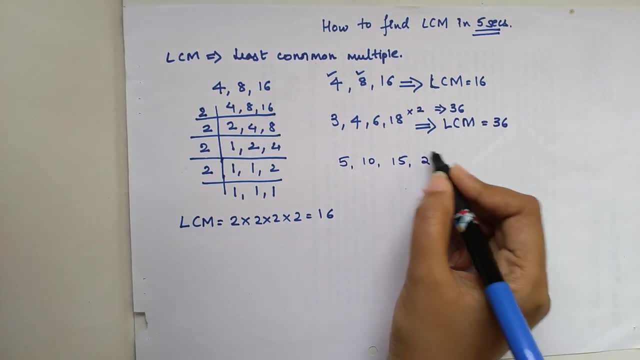 and 20.. As we know that the highest number is 20, and 20 does come in 5's table And it also comes in 10's table, but it does not come in 15's table. So the next step which we do is we try to multiply it with 2.. 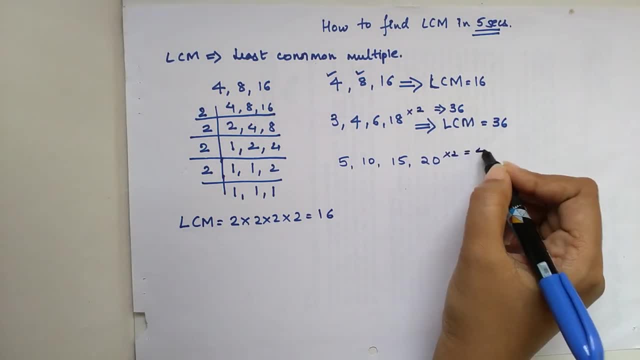 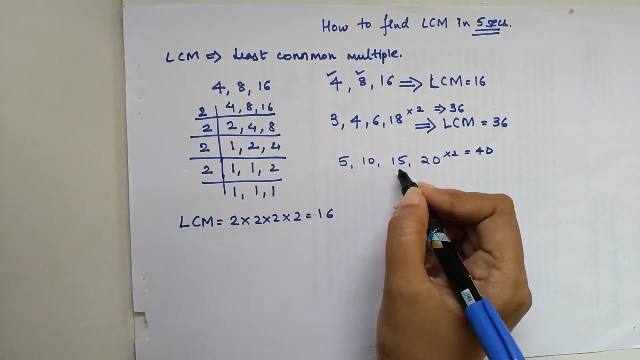 So the answer which we get is 40. Again, does 40 go in 5's table, 10's table and 15's table? It does go in 5 and 10's table but does not go in 15's table. 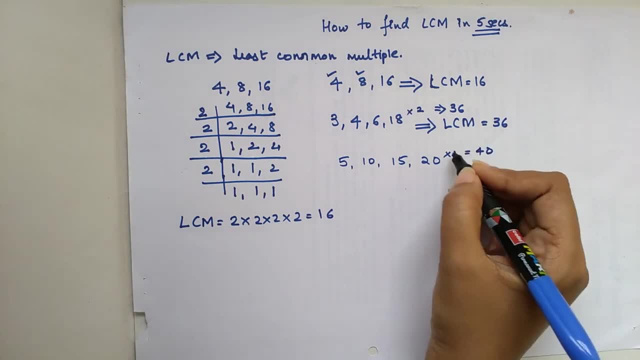 So over here, what do we do? We cancel this and we multiply 20 by 3.. So 20 into 3 gets us 60. Now check whether 60 is coming in 5's, 10's as well as 15's table. 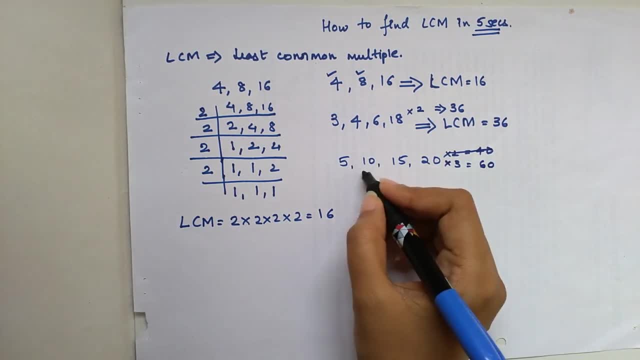 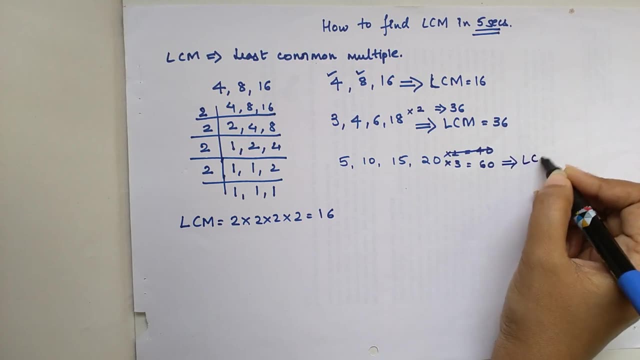 Yes, right, 5 12s are 60, 10 6s are 60 and 15 4s are 60. So here my LCM became 60. Now let me show you another example with prime numbers. 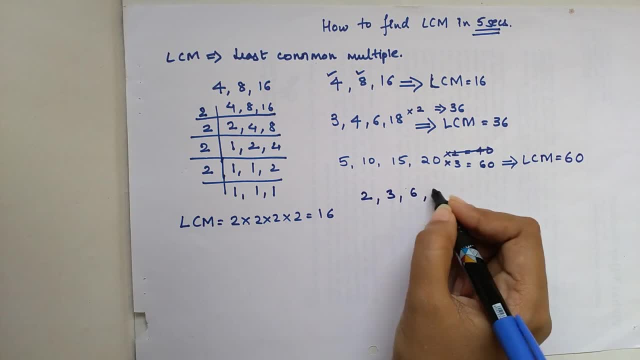 So the numbers are 2,, 3,, 6,, 7 and 12.. Again, we'll check whatever is the highest number. The highest number is 12.. And we can say that 12 comes in 2's table. 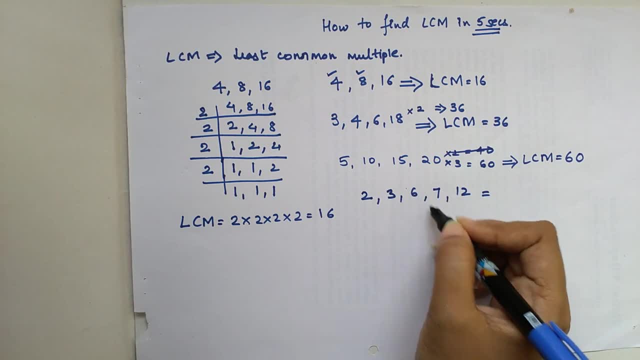 it comes in 3's table and it comes in 6's table, but it doesn't come in 7's table. Now, the problem over here is that 7 is a prime number. So if you use the same trick and you try and multiply 12 into 2,, 12 into 3,, 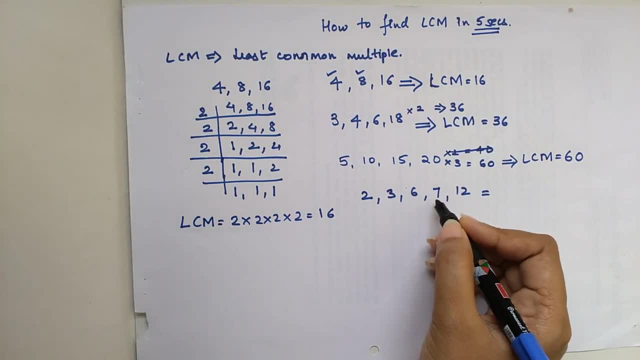 still, your answers would not be a multiple of 7.. Why The reason being? 7 is a prime number. So in such a case, when the highest number is not a multiple of any of the other prime numbers given, then what you need to do is you need to simply multiply the highest number. 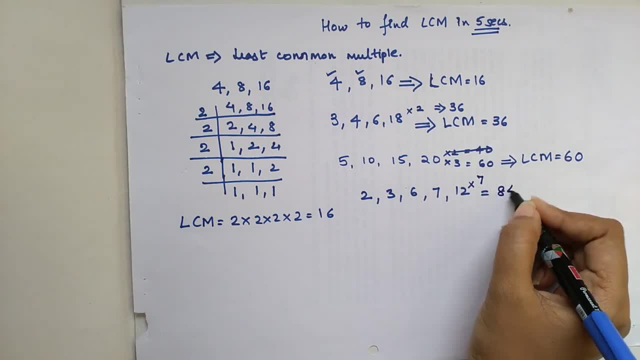 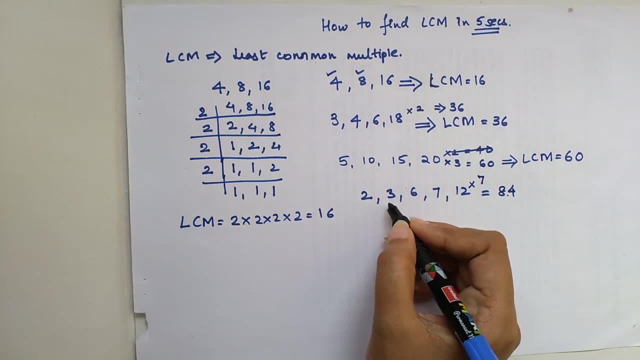 by that prime number. So 12 into 7 is 84. Now let us check whether 84 comes in 2's table- Yes. Whether 84 comes in 3's table- Yes. Whether 84 comes in 6's table. 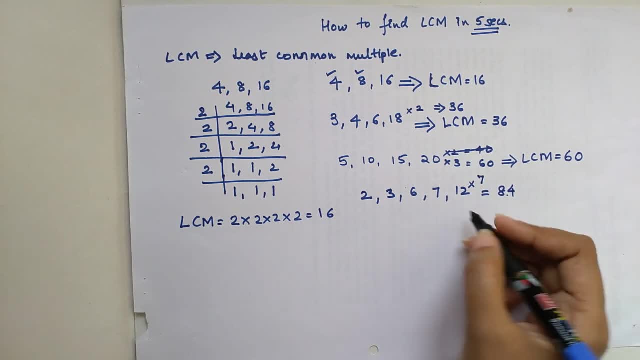 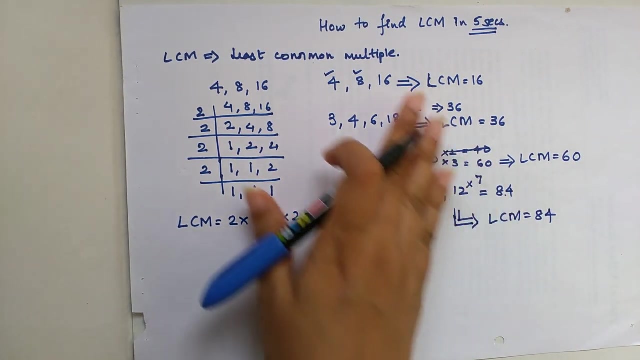 Yes, Whether 84 comes in 7's table, Yes. So here now I can say my LCM has become 84. So let's just revise quickly. Whenever we are given a set of numbers, what do we do? We first pick out the highest number and we check whether that number is a multiple. 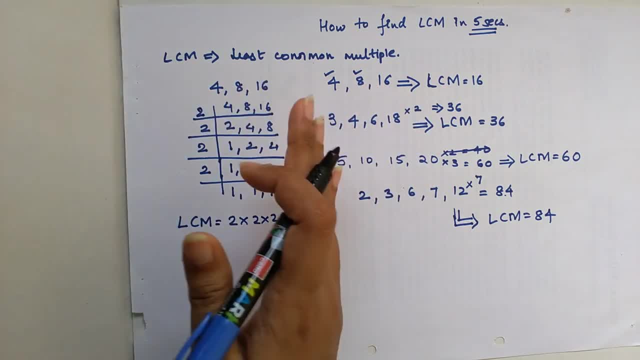 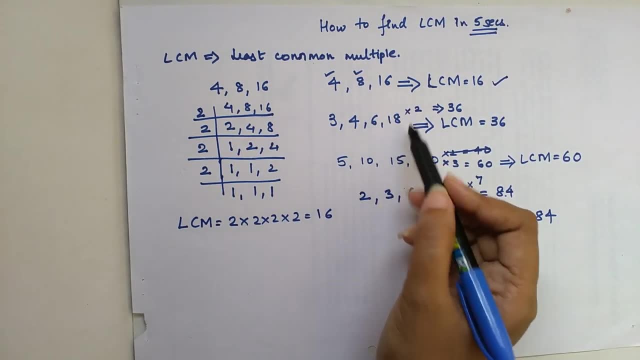 or it comes in the table. So in this case it is a multiple of all the other numbers. If it does come, then that number itself is my LCM, like in my first scenario. Now, if the number given is a multiple of few numbers but not all the numbers,